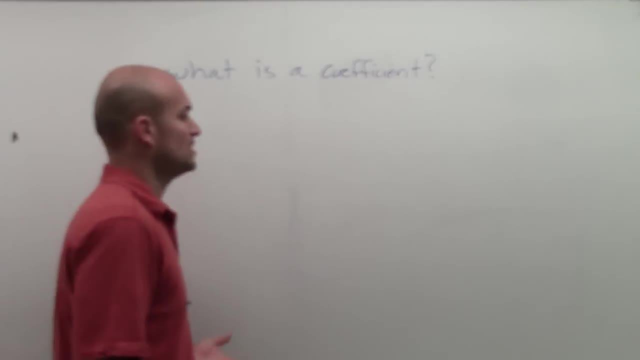 All right, what is a coefficient? So so far we've been talking about terms: variables, constants, right? So here's x. That's what we call a variable. When a number is not being multiplied by a variable, we call it a constant. 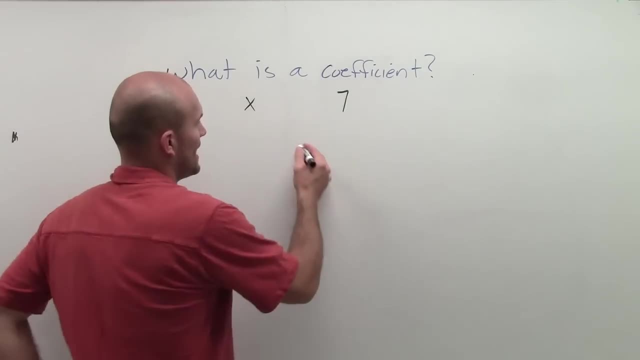 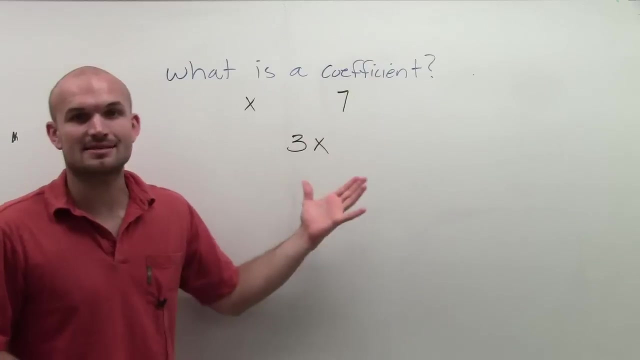 So we have a variable and a constant. They're both terms. But then what happens when we have a term that's like 3x, right? Well, it has a variable part of it and it has a constant part of it. 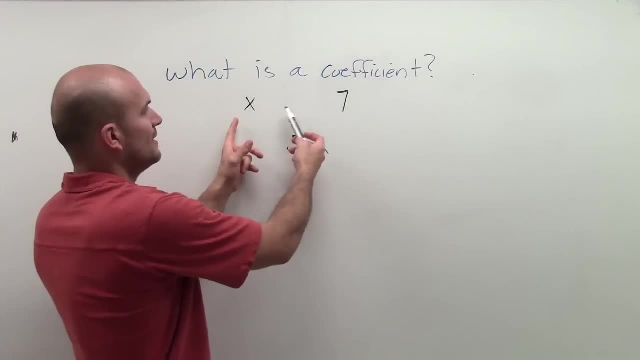 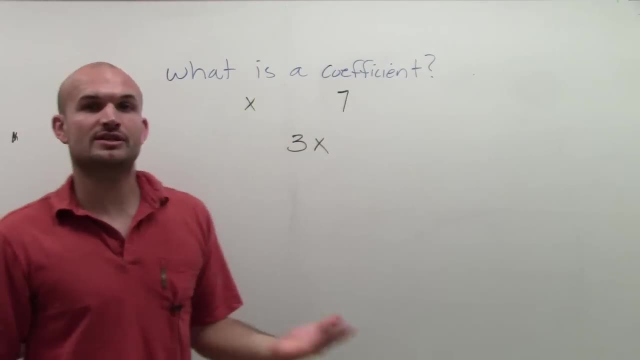 But there's another special part of when we combine a number and a variable together, we also now develop what the coefficient is. So the coefficient is going to be your numeric factor of that term, which is going to be pretty much the number in your term. 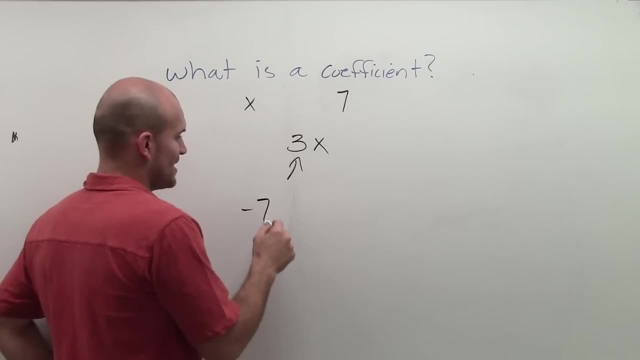 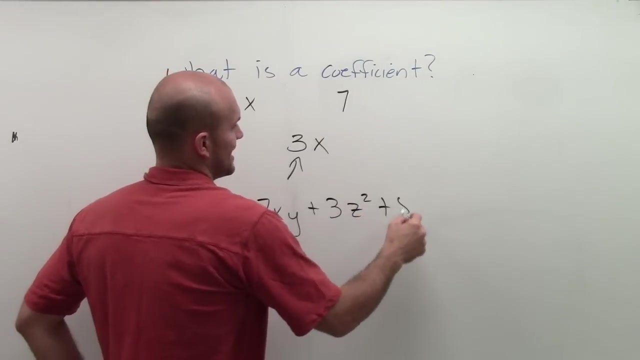 So that's going to be 3x. So let's just write out something. Let's say negative 7xy plus 3z, squared plus 8, all right. So if I want to say What are all of my coefficients? right? 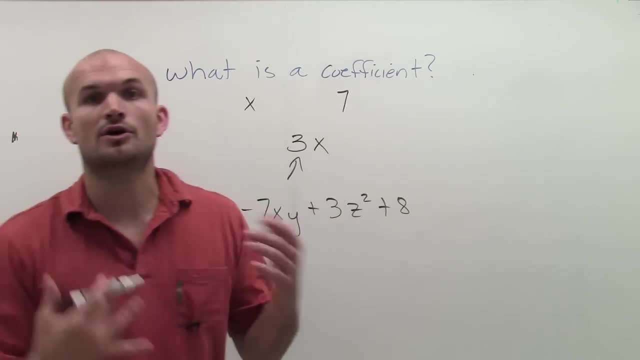 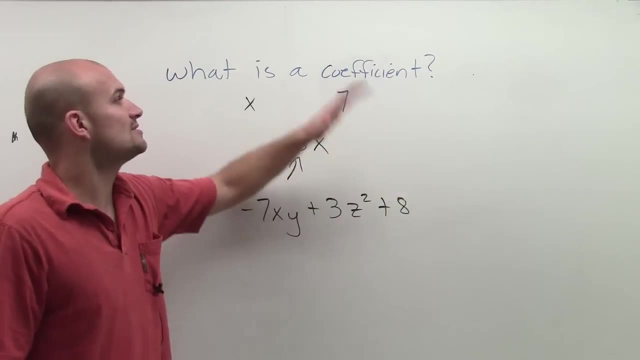 And a lot of times your teacher will say, hey, take your coefficient, or here's the coefficient of this value. So let's look at all the coefficients. Well, 8 is a constant, so it doesn't have a variable with it. 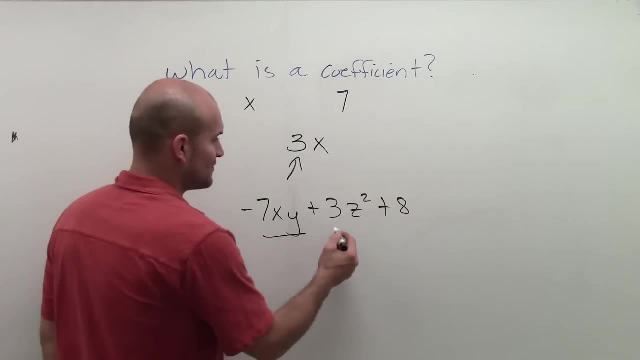 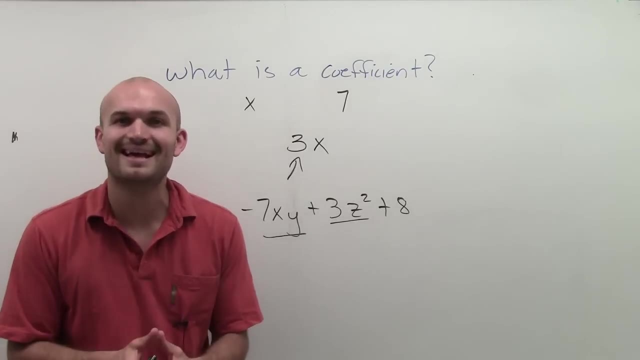 So it's not going to have a coefficient. So my only two terms that can have coefficients are these two terms. And remember, your coefficient is your numeric term. It is your numeric term, Your numeric factor of your term. So let's look at what is the number that 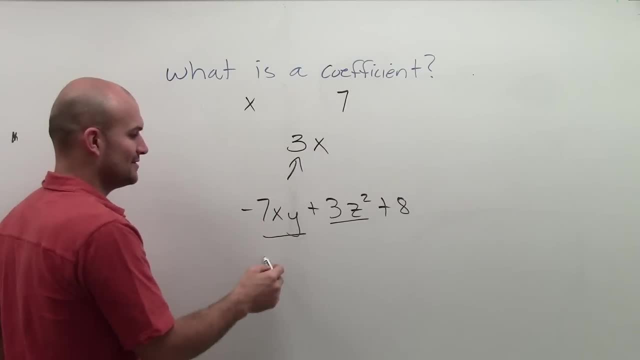 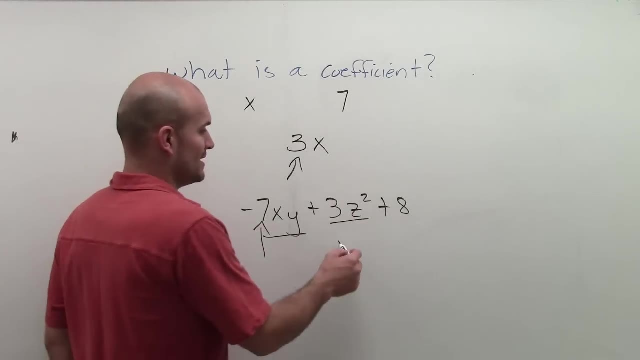 is going to be my factor. Well, my two variable factors are x and y, so the number is negative: 7.. Here, my variable factor is z, squared, The number factor is 3.. Because, remember, factors are your numbers that multiply to give you your term. 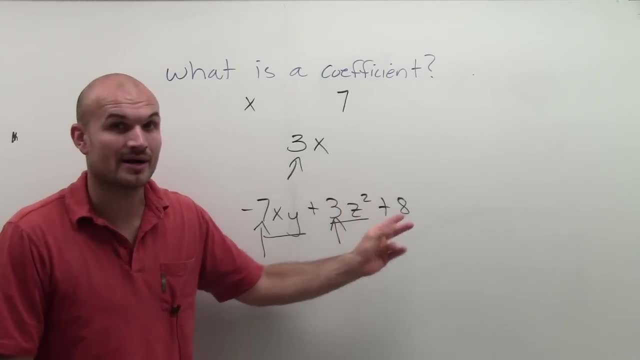 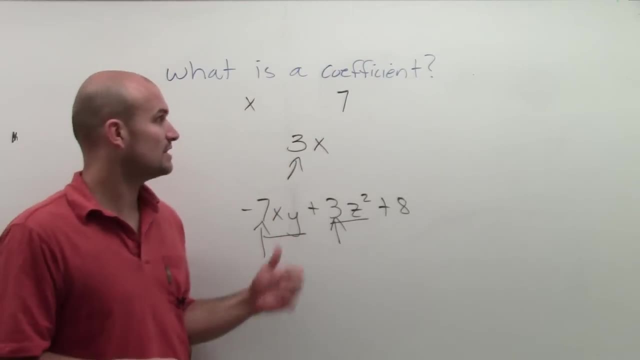 Well, the two terms that my two factors are 3 and z, squared, The number factor is 3, so that is my coefficient, As is 7 is my coefficient for this term. So that is a brief little description of what the coefficient is. Hope it helps.